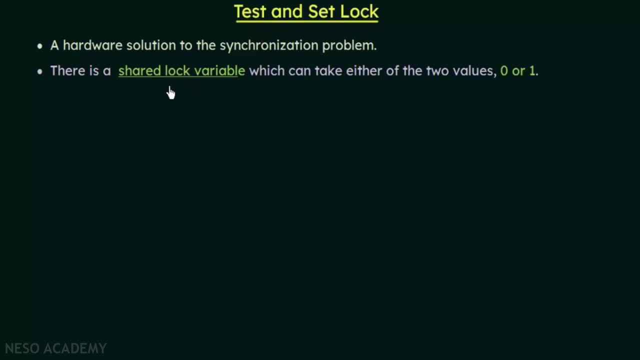 So the main thing in this test and set log is this log variable, which is a shared variable, which is shared between different processes. So this log variable will have two values, which can be either 0 or 1.. So if the value is 0 means it is unlocked and if the value is 1 means it is locked. 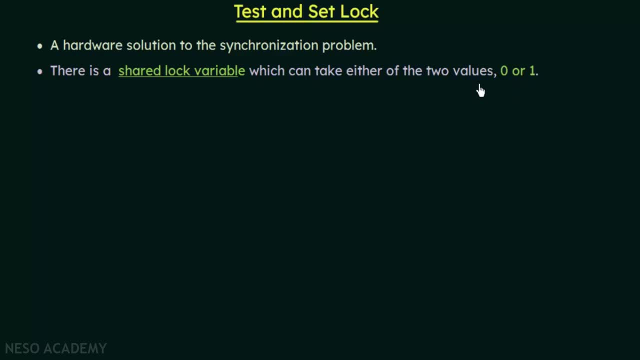 So if the shared log variable has the value 0, that means the lock is unlocked, and if it is having the value 1 means it is locked. Now what happens is, before entering into the critical section, a process inquires about the lock. 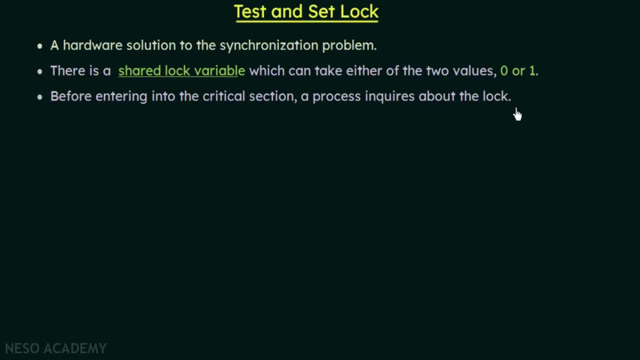 So when a process wants to enter its critical section, what it will do is it will inquire about the lock. It will see whether the lock's value is set to 0 or 1. So it wants to find out whether it is locked or unlocked. 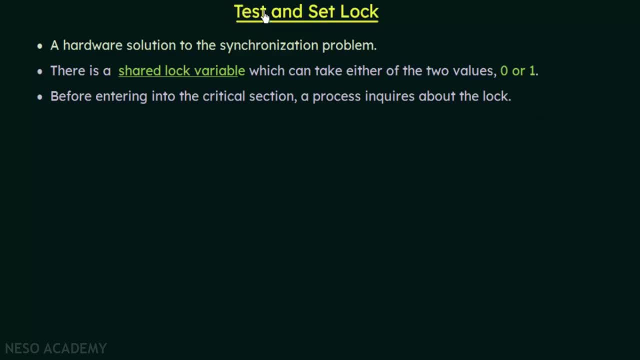 So that is the testing part. So let's try to understand the name. So the testing part is what we saw here just now. So when a process wants to enter its critical section, it will inquire if the lock variable is 0 or 1.. 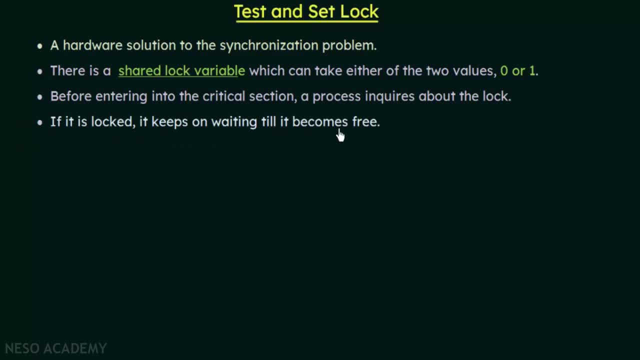 Now, if it is locked, it keeps on waiting till it becomes free. So when a process wants to enter its critical section and when it inquires about the lock and if it finds that the lock value is set to 1, which implies that it is locked, then 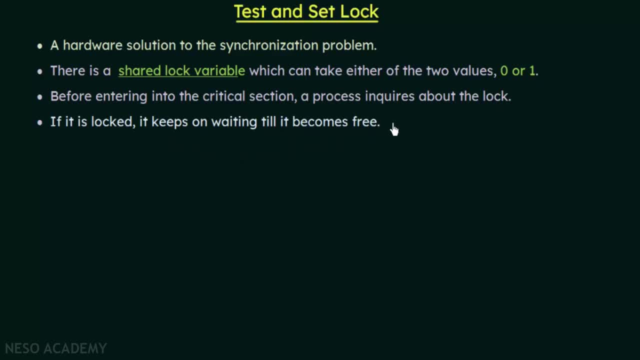 what will it do? It will keep on waiting until it becomes free. So when the lock value is set to 1, or when it is locked, it implies that some other process is currently executing in its critical section, and so no other processes should be allowed. 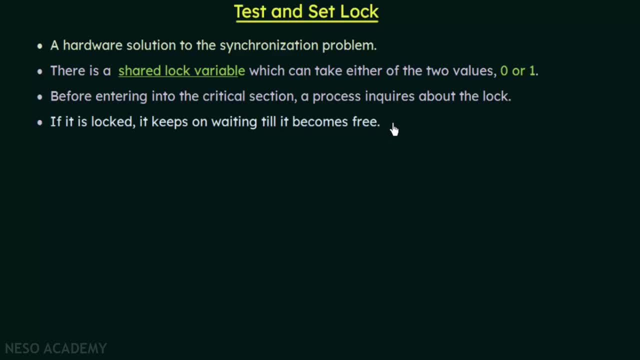 to enter its critical section at that time. So that is what we mean by this lock. So if it is locked, it will have to keep on waiting until it becomes free, And then, if it is not locked, it takes the lock and executes the critical section. 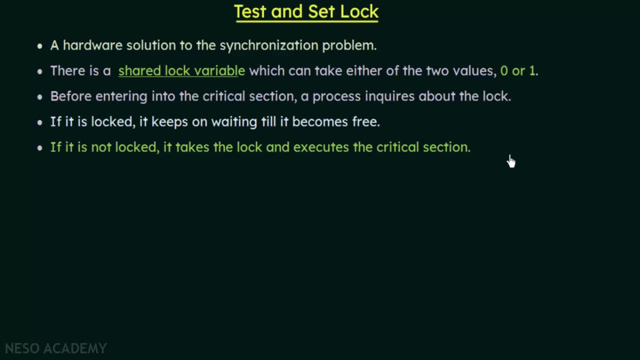 So if it finds that the lock value is set to 0, that means if it is unlocked- then the process will take the lock and set the lock value to 1.. So that is what we mean by this lock. That means that process will set the lock and then it will execute in its critical section. 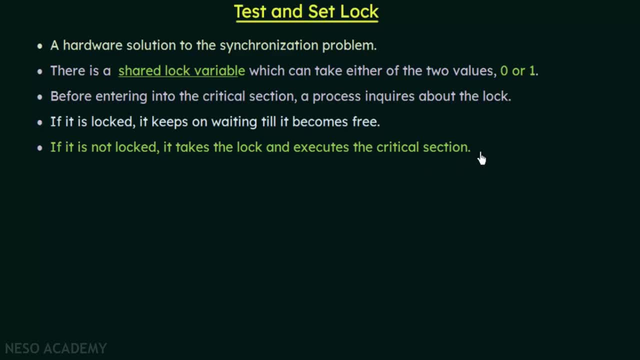 So this is the basic idea. So in a nutshell, we can just say that when a process wants to enter its critical section, it will have to first check the lock, and if the lock is found to be locked, then it has to wait, and if it is unlocked, then it can take the lock and set the lock and then execute. 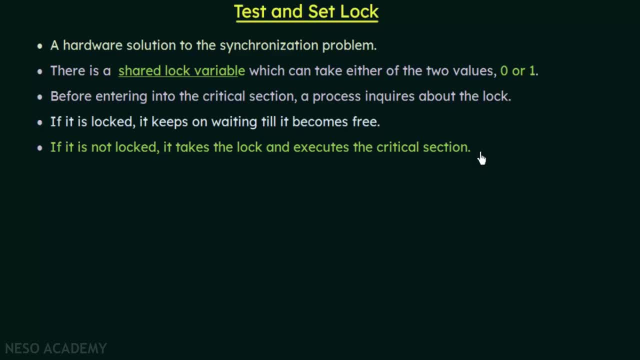 in its critical section. So the lock variable is shared between the different processes. It's a shared variable. So let me just take a simple real life example. Let's say that there is a room which can be used by only one person at a time. 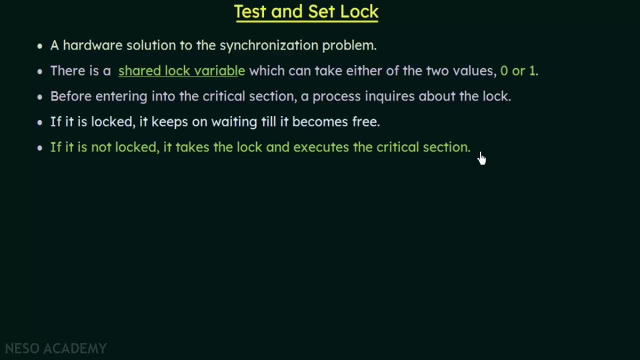 So when a person comes, he checks whether the room is locked or unlocked. So if it is unlocked he can open the room, go inside the room and he will lock the room from inside and he will do his work. So if another person tries to enter the room at that time he checks if the room is locked. 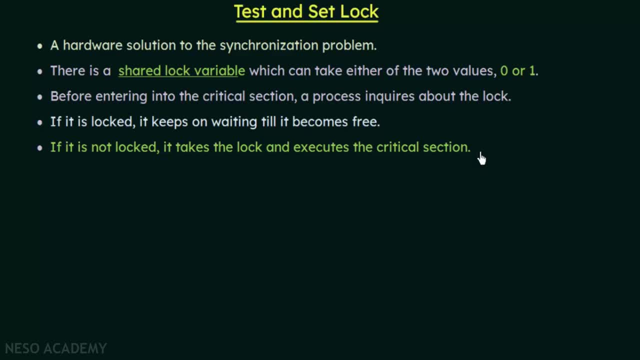 and finds that the room is locked So he cannot enter at that time. If the person who is currently in the room finishes his work and comes out, then only the next person can enter the room when the room is unlocked. So this is the simple concept of this test and set lock. 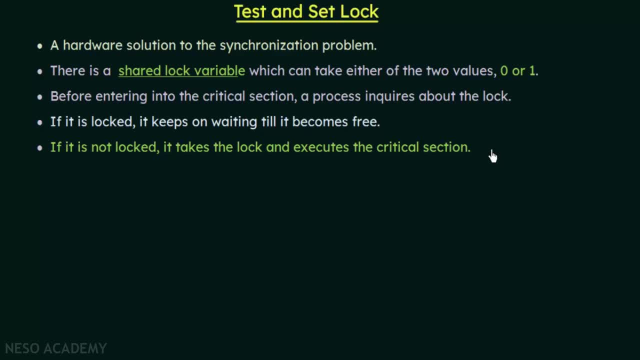 So that is what happens here. Now, since we have a basic idea of how it works, we will see the underlying design of this test and set instruction and we will be seeing how it is implemented when processes tries to enter in their critical section. So here we have the definition of the test and set instruction. 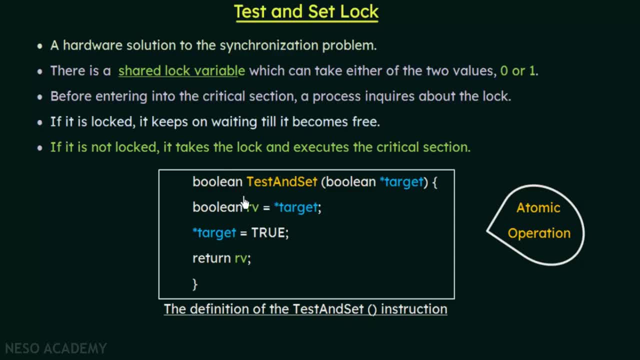 So this test and set instruction is nothing but a function, and this function has a Boolean return type. So Boolean return type means this function will return a variable which is of Boolean data type. So what is a Boolean data type? A Boolean data type is a data type that can take only two values, like, for example, zero. 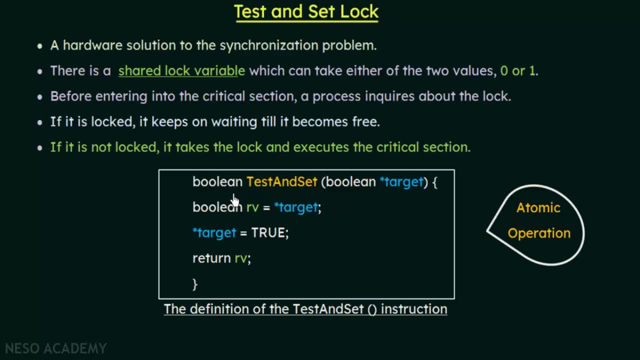 or one, or true or false and so on. So that is a return type of this function and also this function takes a Boolean variable as an argument. So the argument that is taken by this function, that is, this target variable, is also a Boolean data type. 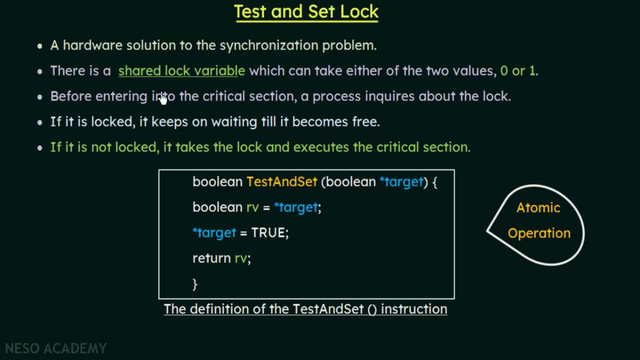 So this target variable will signify the log variable. So we said that there is going to be a shared log variable. So this log variable's value will be passed to this target variable over here. So it will have either zero or one as a value. 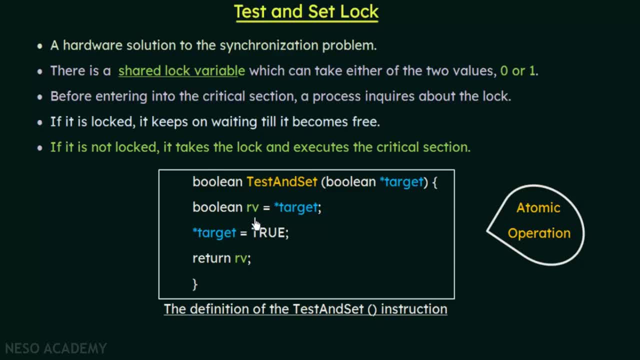 And now, inside this function, what happens? we are having another variable called rv, which is also of Boolean type, And then we have a Boolean data type And then we are storing the target's value to this rv. So if target value is zero, then rv value will also be zero. 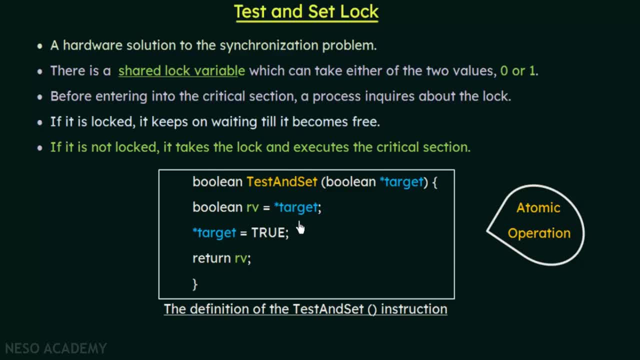 If target value is one, rv value also will be one, And after that we are setting the target value back to true again and then we are returning the value of rv. So whatever is passed to this function, that is, this target variable will be the one that 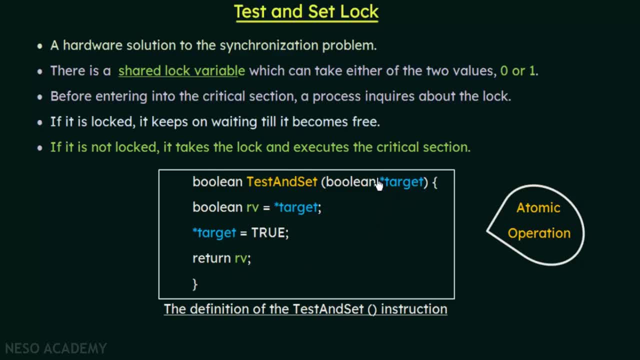 is going to be returned. Why is that? Because that target variable is stored into rv And that exact thing is what is going to be returned. All right, So this is what happens. And then here I have written something called atomic operation. 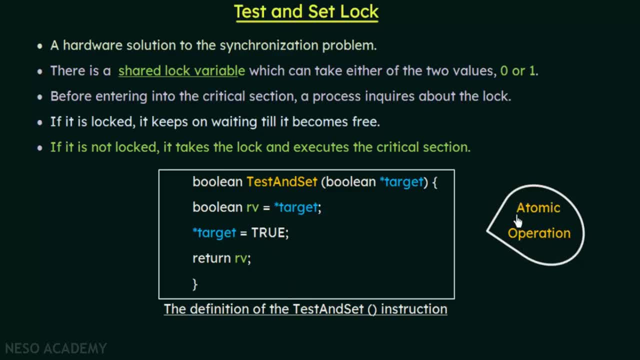 So what do we mean by this? I have written this atomic operation because in this test and set log instruction, whatever is happening in a process, that is, when a process checks for the log and if the log is available, and when it acquires a log and sets the log value to one and executes in. 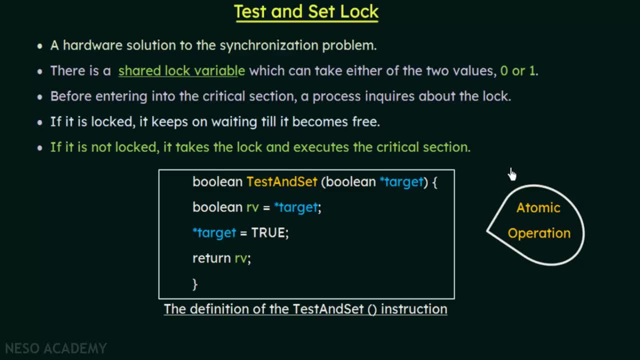 its critical section. All this is going to be returned, But this task will happen as a single operation which cannot be interrupted by anyone. So that is what we mean by atomic operation: It is a single operation that will be uninterrupted. So keep in mind that whatever is happening in this test and set log when a process acquires- 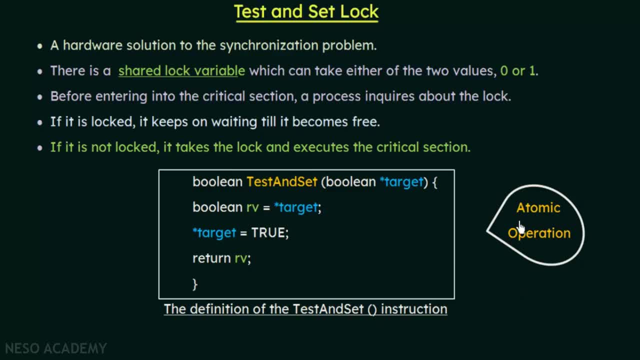 a log and executes in its critical section, it will be happening as an atomic operation, All right, So keep that in mind. And here we have seen the definition of the test and set instruction. And now let us see when a process wants to enter this critical section, how does this? 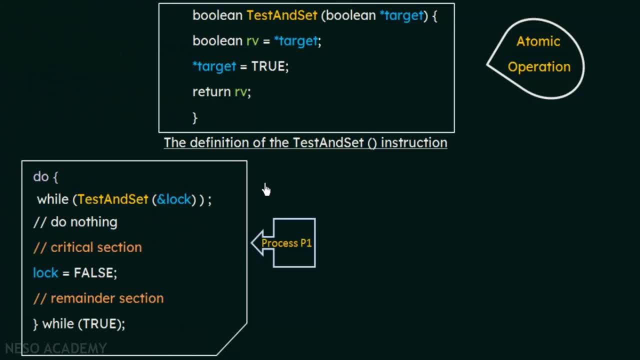 work. All right. Here we have the structure of a process, which we will call process P1, which wants to enter its critical section. So here we are going to make use of the test and set log in order to achieve process synchronization. All right. 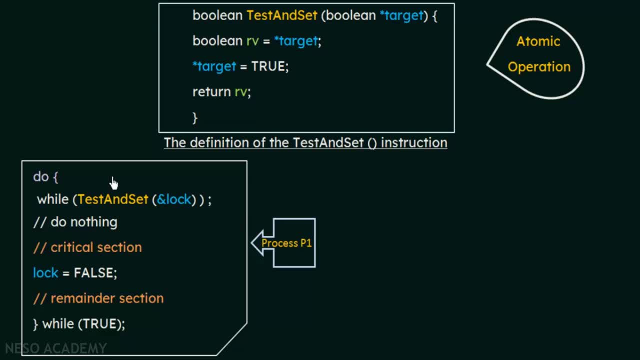 So let's see So this process P1, it wants to enter its critical section. So what it will do, It will come to this do while loop. So in this do while loop, We have the test And set function, And then the log variable is passed to the function. 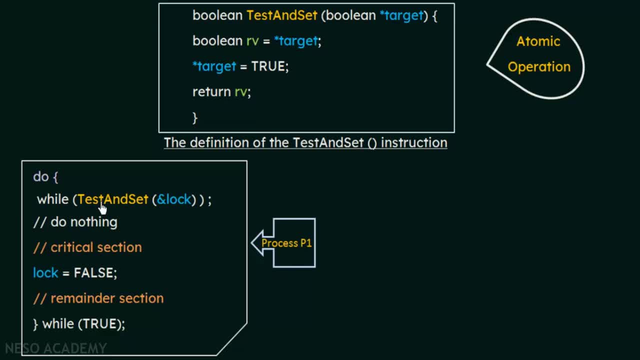 Okay, So when this process P1 wants to enter its critical section, it will come to this do while loop And in this, do while loop. what are we having in this while condition? Let's see: Inside this while loop, we are having the test and set function, which is this function: 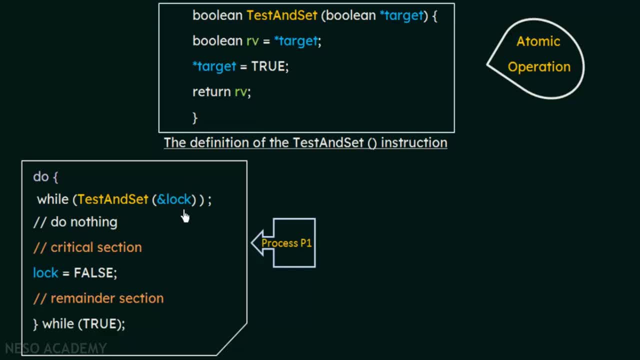 And then we are passing as an argument the log. So the log variable will always be set to zero in the beginning. So keep in mind that the log value is always zero initially. So here we see that we are actually passing the address of the log ampersand log. 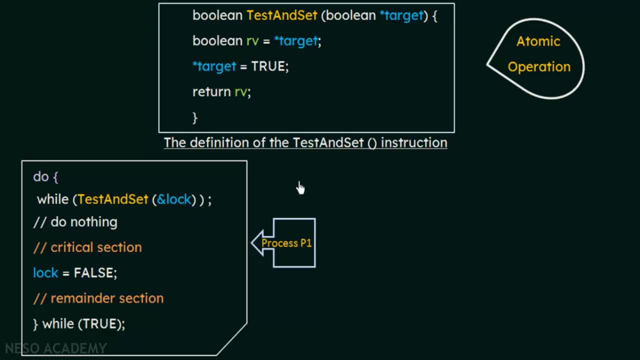 And here we are actually using a pointer variable. So we are using this in this way because, as I told you, this log variable is shared between different processes, So we need to have the current value of this log every time process accesses this log variable. 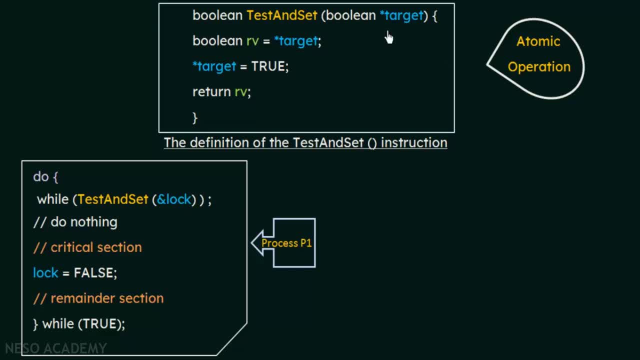 That is why we are making use of this address and pointer and all, So you don't have to get confused. going to the detail of the code, Just understand that this is a shared variable. That is why we are going to make use of the address and pointer and all that. 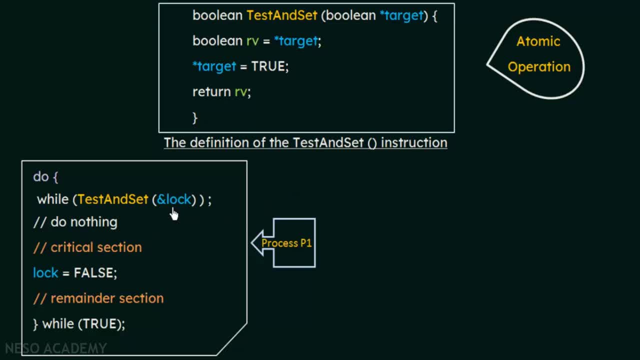 So, for simplicity, just remember that it is a shared variable and we are going to treat it as a normal variable. Okay, So let's see. As I told you, the log's value is set to zero, always in the beginning. So when process P1 wants to enter this critical section- assuming that this is the beginning- 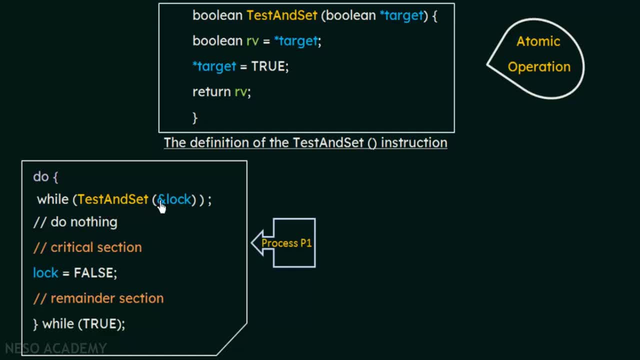 the log's value is zero. So we have test and set, and instead of log we have zero. So test and set of zero is called. Now where is test and set? This is the definition of test and set, and we have a Boolean target here. 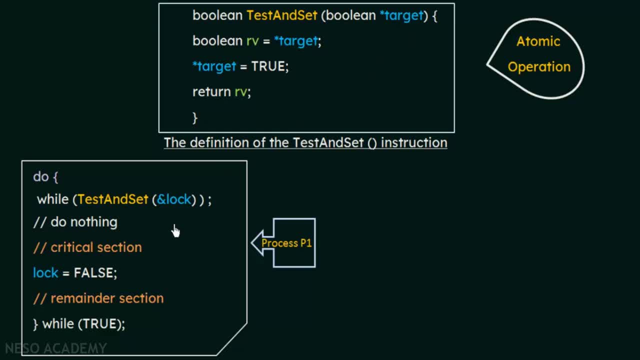 So whatever is passed from here will be stored in this target. So here we passed zero, So the target's value will be zero. Now what will happen? We come into this function and we have a Boolean RV and it is equal to the target. 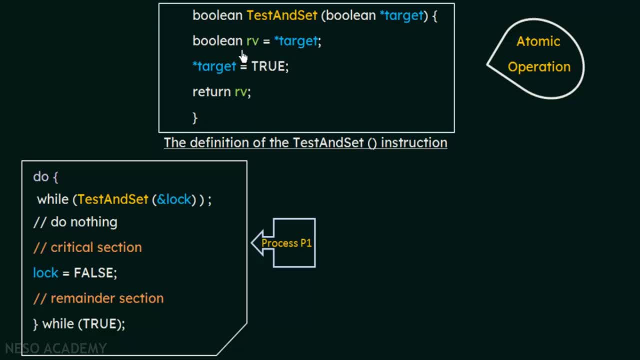 That means whatever value is there in target, we are storing it to this RV. So what is target? It is zero. We got that zero from here, So this value of target is zero now. So target's value is stored to RV. 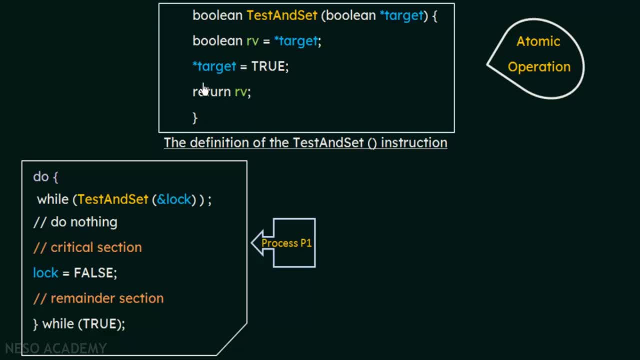 So RV's value also is now zero. and then the target value is set back to true. again, Target is equal to true and then return RV. So what is RV? RV is zero, I told you. So RV is going to be returned. That means zero is going to be returned. 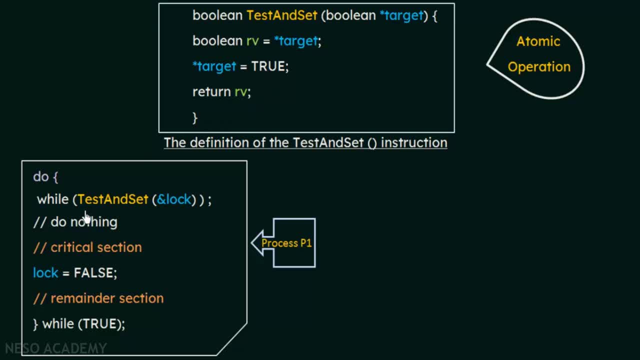 So this whole function is going to return the value zero. So when we call the function here Passing the value zero, zero is returned. So the result of this entire function will be zero. So it is like while This whole thing becomes zero. 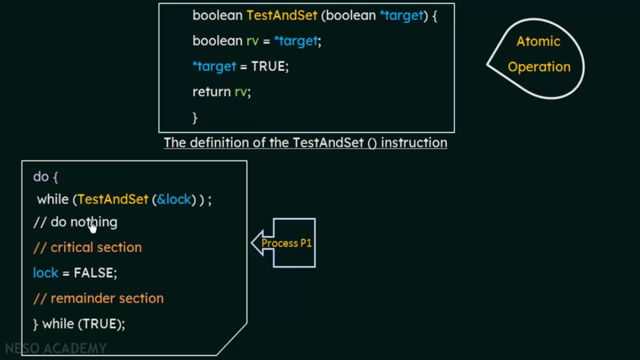 Now look at this while loop again. there is a semi colon here. That means there are no instruction inside this while loop. We are only having the condition and as long as the condition is true, the control will remain inside this while and it will continue looping inside this while As long. 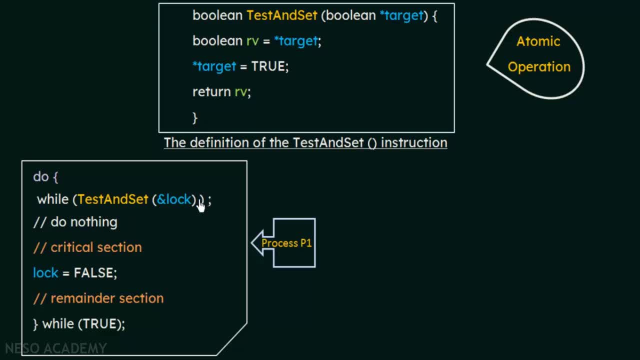 as the condition is true, and when the condition becomes false, it will break out of the while loop and come to the remaining part. Now, here, as I told you, the return value was rv, which is zero, so it becomes while zero. So keep another thing in mind: in the while loop, when we are having the 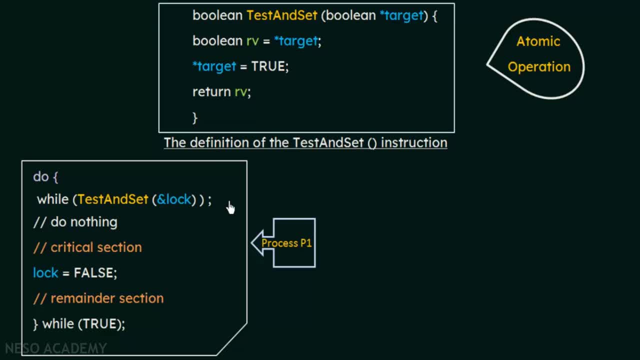 value one, that means the while condition is true, and when we are having the value zero, the while condition will become false. Okay, that is the concept of while loop. So here we know that zero was returned, so it becomes while of zero. So while of zero means what While condition becomes. 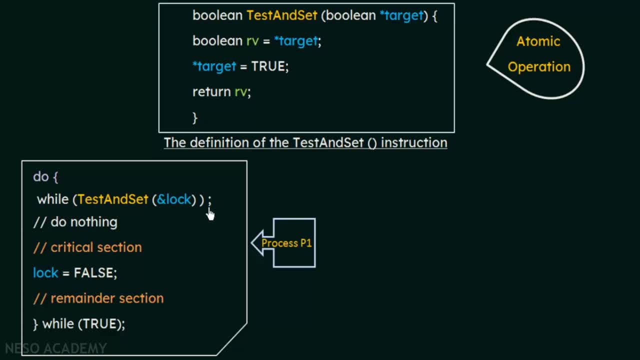 false. So when while condition becomes false, it will break out of this while loop and it will come to the critical section. So it comes to the critical section and it will execute in its critical section. So why is it able to execute in its critical section? Because the log value was: 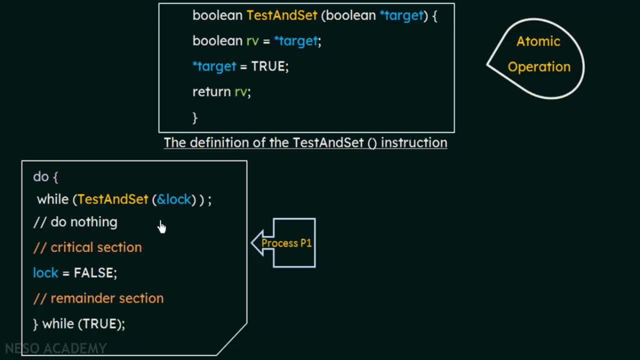 initially set to zero, So zero implies that no processes are currently executing in their critical sections. So that is why this while loop was able to break and it came to the critical section and it is executing in its critical section. and while it is executing in its critical section, what is the? 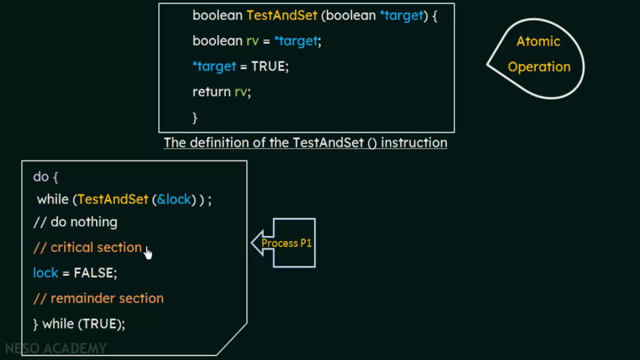 current value of log at that time. That also we need to keep in mind. So we see that log and target, as I told you, is going to be the same thing. So target value, if you look here, was set to true. So after this log became false and enters this critical section, 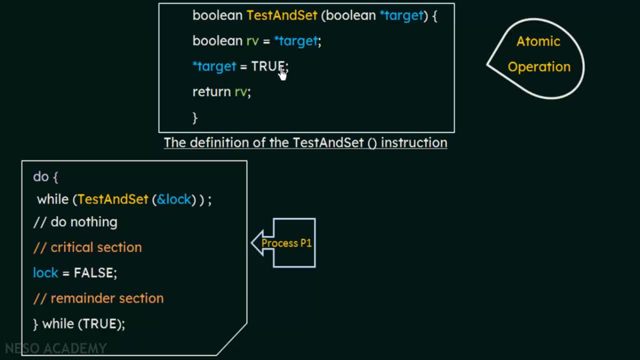 at that time the target value is also set to true. That means the logs value is again set to 1.. So while it is executing in its critical section, the logs value is currently 1 and at that time no other process can enter the critical section. So after the critical section of this, 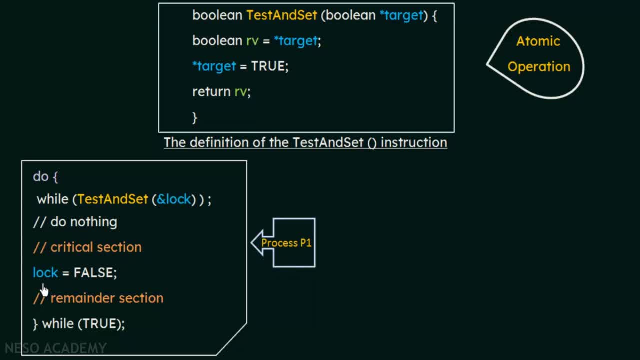 process P1 is completed, then it will again set the log value as false and then execute the remainder section. So when it sets the log value as false, at that time the process will come to typical locationr betrayal will detect a mistake later. So we must create this log by stopping on implies n-sets to 1.. So we need to make change of the backgio. Now again we are not going to use the log. So once again we can set the log value as false and enter the critical section and at that time�. 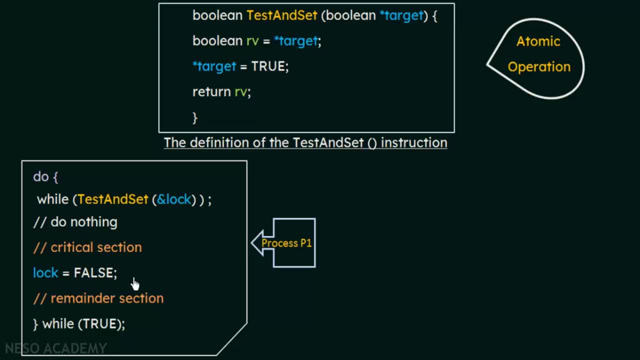 the log value as false- false at this point of time. if there are any other process that wants to enter its critical section, then they will be allowed to enter their critical section because the lock is now set to false. all right, so this is how it works in process p1. now let's go a little backward and 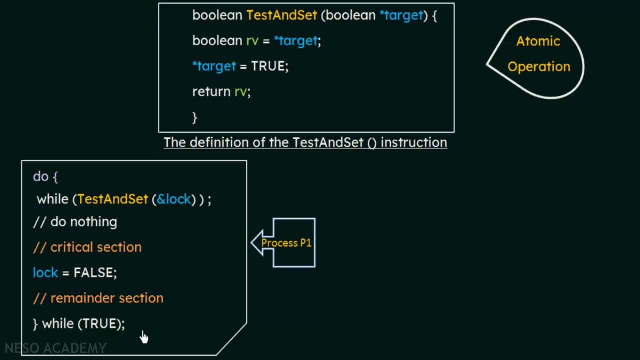 let's say that there is another process, p2, that tries to enter its critical section when p1 was actually already executing in its critical section. so here we have a process p2 that tries to execute its critical section, so it will also do the same thing. so it has its own while loop and it is going. 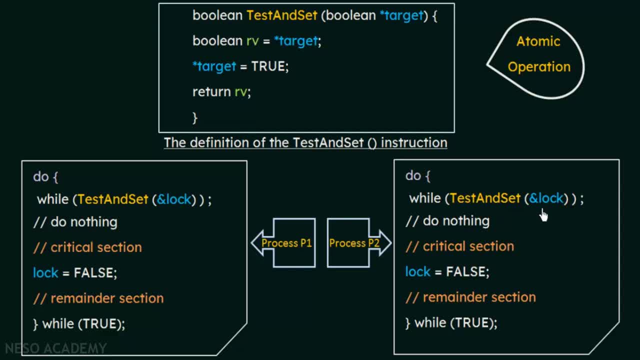 to call the test and set instruction with the value of the lock. now, here is the most important thing: what is the value of the lock? now, i told you, the locks value is set to one when it is executing in its critical section. here we already set the target equal to true, and after that only we broke. 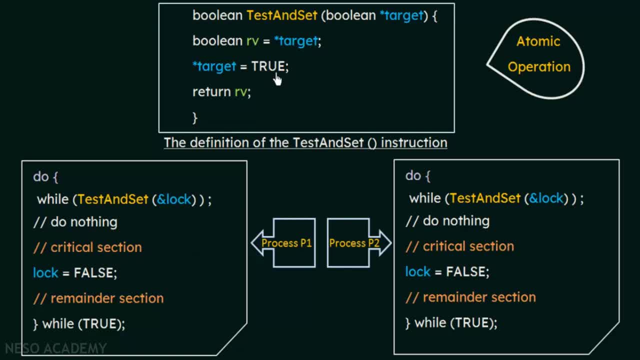 from the loop and came to the critical section. so the target's value is true means the locks value is one. so here the logs value that will be passed will be one. so it says test and set of one. so when test and set of one is called, what will happen? one will be passed to this target variable. 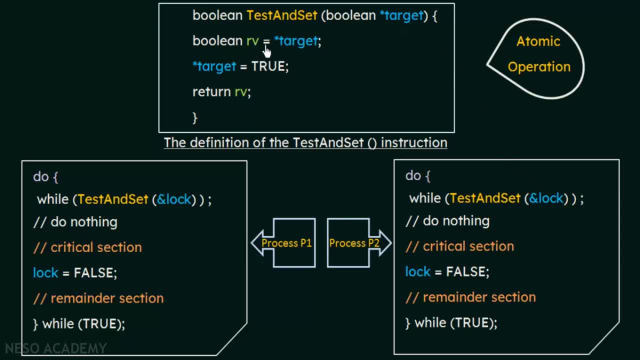 now, when one is passed to the target variable, what happens? rv is equal to target. that means rv also will be equal to one. then target is set to true and then return rv. so what is rv? rv's value is one, so one is going to be returned in this function. so here, one is set to true and 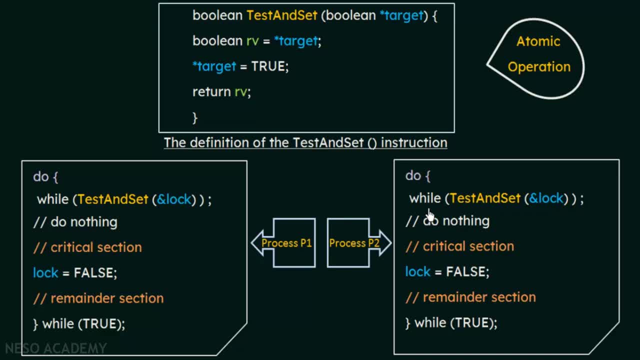 so. so here one is going to be returned when this function is called, and so it is going to be while of one. this entire thing becomes one and, as i told you in while loop, when the condition is one, that means the while condition is true, and when the while condition is true, it will keep looping. 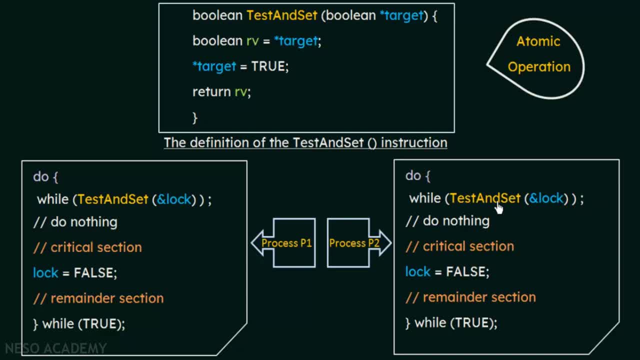 inside the while loop and it will not come out of the while loop because of this semicolon. so, since it is one, it will stay inside this while loop and it will do nothing but inside the while loop and it will not come to this critical section part. So we see that when p1 is 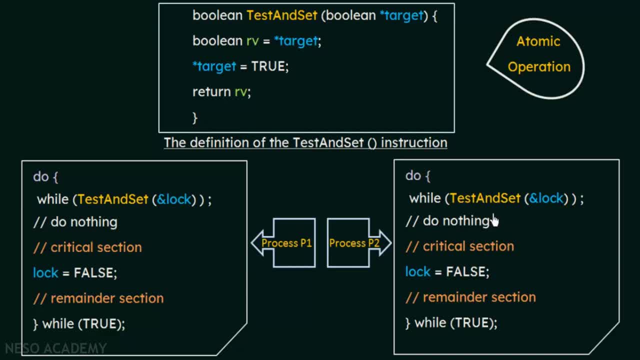 executing in its critical section. even though p2 tried to enter the critical section, it cannot enter its critical section because of the way it is designed. Alright, now let's say that p1 completed its execution of critical section and at that time it will set the log value as false. 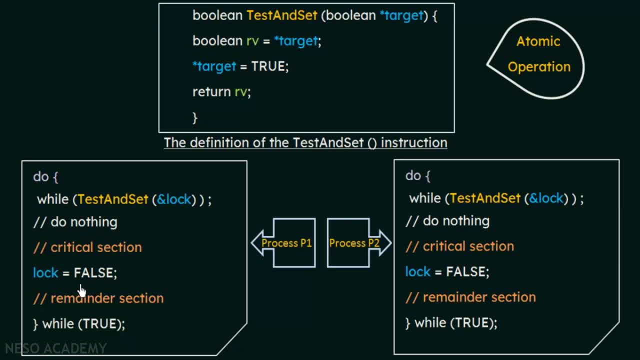 or 0.. Now, when the log value is set to 0, what happens if p2 is still trying to execute in its critical section? So here the log value now becomes 0 because it is set to false here. So 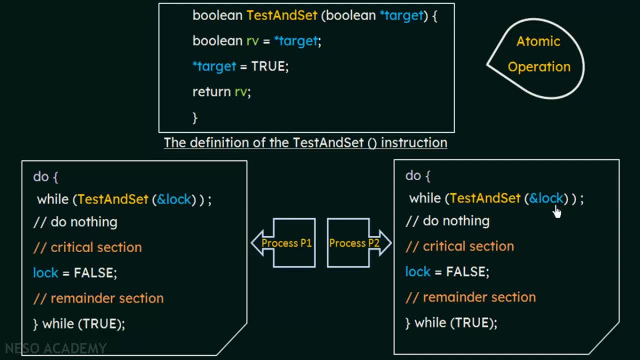 false and 0, same thing. So it is set to 0.. So it becomes 0, and when test and set of 0 is called, we know what will happen here: Target becomes 0 and rv is equal to. target means rv is equal to 0.. 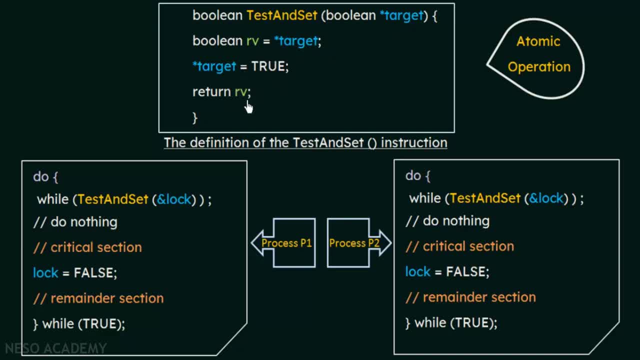 Then target is set to true and rv is returned, which is 0. So 0 gets returned over here. So this whole value becomes 0. and when the whole value becomes 0, what happens? The while condition becomes false. and when while condition becomes false. 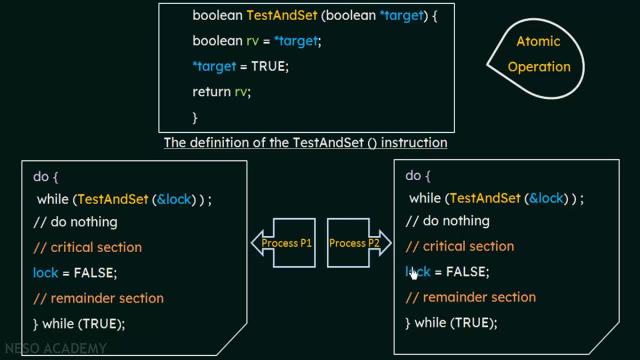 it will break out of the while loop and it will come to the critical section and it will execute in its critical section. Now, when this is also executing in its critical section, remember that the target is set to true, So the log is set to 1 again and any other process that tries to enter. 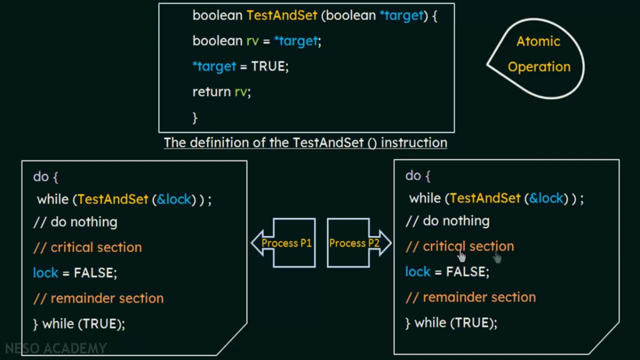 its critical section will not be allowed Because of that, and then, after this P2 completes its critical section, it will set the log value as false again, allowing other processes to enter their critical sections, and then it will execute the remainder section. So this is how the test and set log works. So we see that when the log's 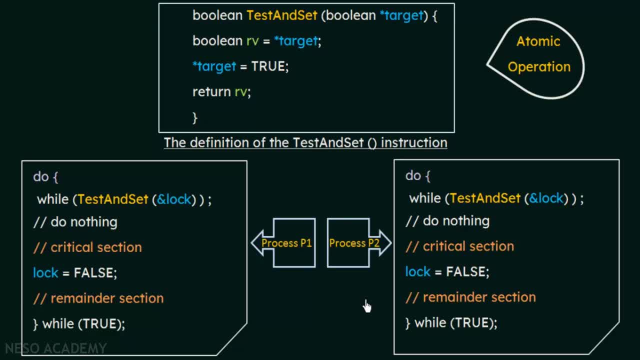 value is 0,, then the process is allowed to enter its critical section and do its execution, and while it is executing in its critical section, the log value is set to 1.. Hence not allowing any other processes to enter their critical sections until and unless the current process finishes its. 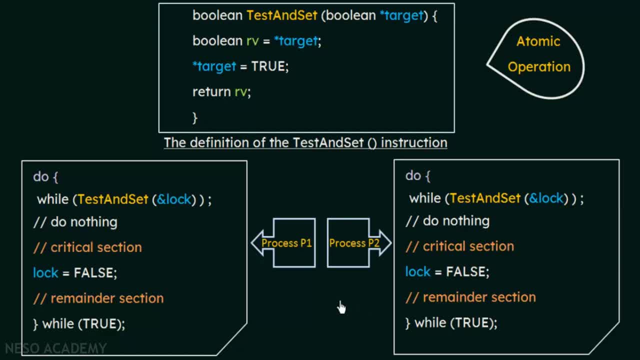 execution in its critical section. So that is how the test and set log is implemented. So keep in mind that this log variable is shared and this is an atomic operation. That means all these things happen as one uninterruptible operation. All right, So this is a hardware-based solution to 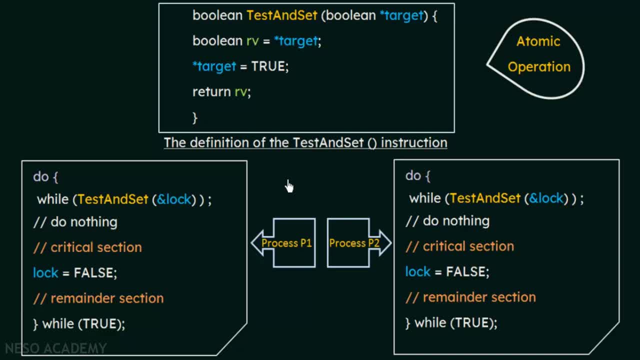 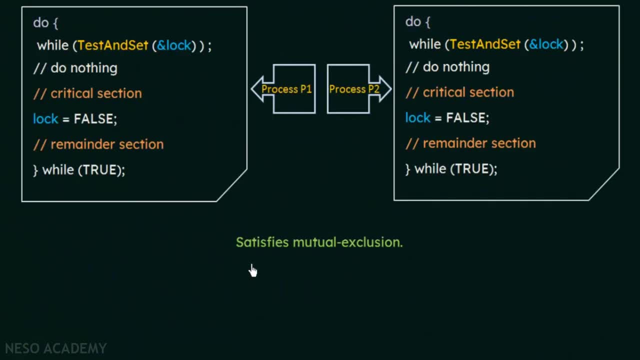 the synchronization problem. and now we have the question if this is the best solution, or does this solution also have any flaws? So let's find out Now. the advantage of this solution is that it satisfies the mutual exclusion. So it satisfies mutual exclusion, I don't need to. 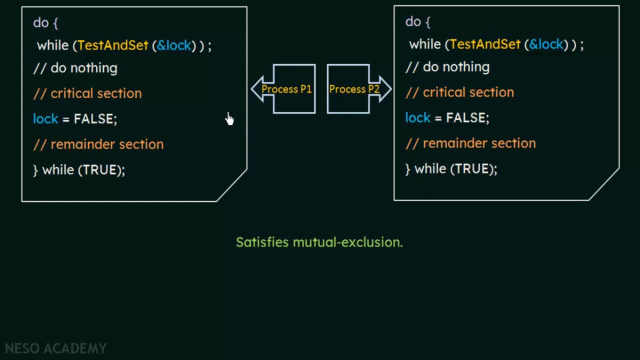 explain it. We have seen it very clearly that when one process is executing in its critical section, the other process is not allowed to enter its critical section. So mutual exclusion is satisfied, but it does not satisfy the bounded weighting. So why is the bounded weighting? 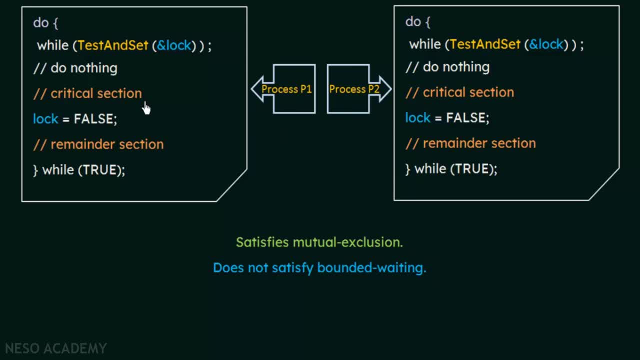 condition not satisfied. So let's say that P1 was executing in its critical section. So P2 tries to execute in its critical section but was not allowed because log was set to 1. and then let's say that P2 was trying to execute for some more time but somehow. 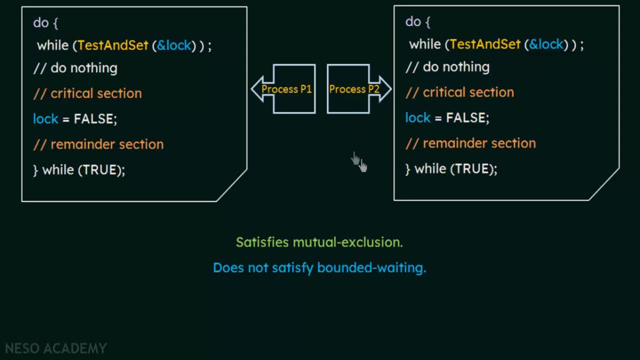 it got preempted and at that time another process, P3- arrived. Now P3 also is trying to enter its critical section, and then it was not able to enter because P1 was already executing. and let's say that at that point of time P1 completes its critical section and sets a log as false. Now P3. 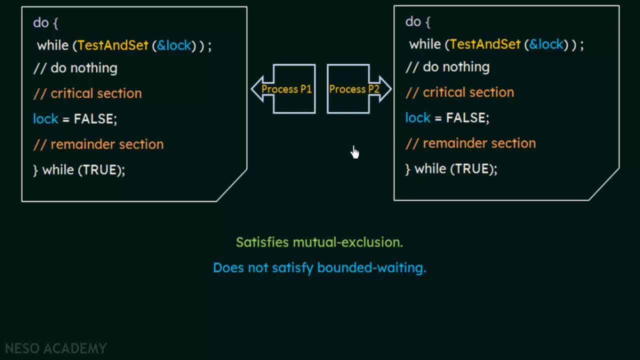 is requesting for the critical section. So, as it is the one requesting right now, it will get hold of the log and it will be able to enter its critical section. So this P2, which is the unlucky process that went away, when it tries to come back and execute in its critical section.